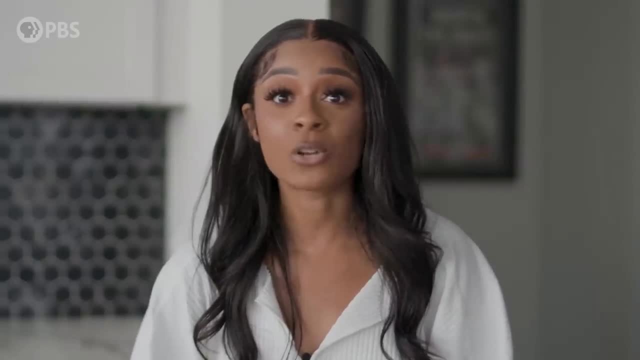 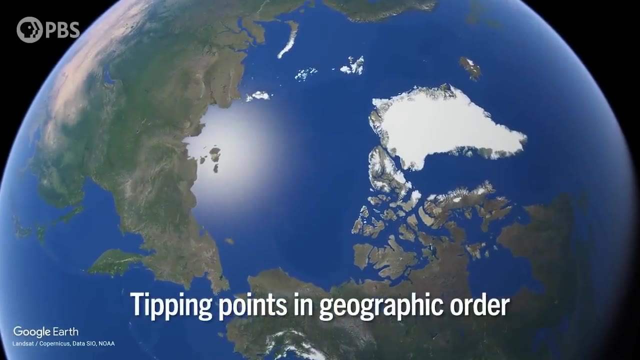 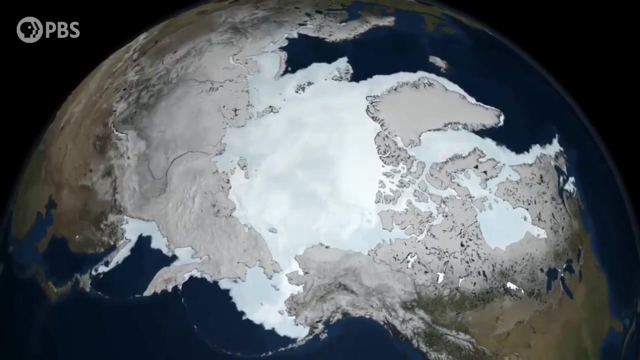 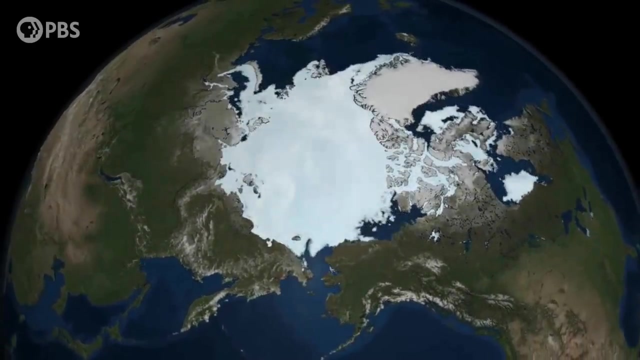 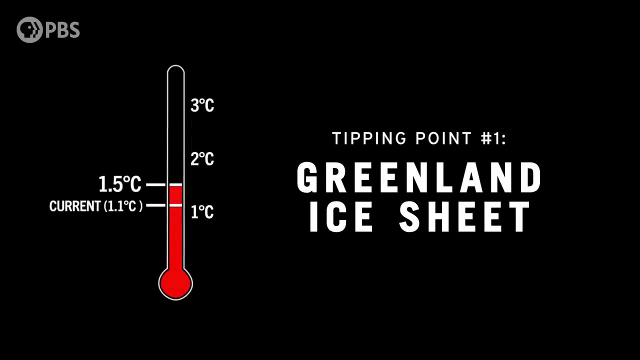 many of our planet's systems getting precariously close to sudden potentially irreversible change. We'll begin our journey all the way up in the Arctic which is warming about two to three times faster than the rest of the planet. This is because as global warming melts the reflective white sea ice more and more of the dark blue ocean below is revealed which absorbs energy from the Sun further warming the region. That gets us to our first tipping point. 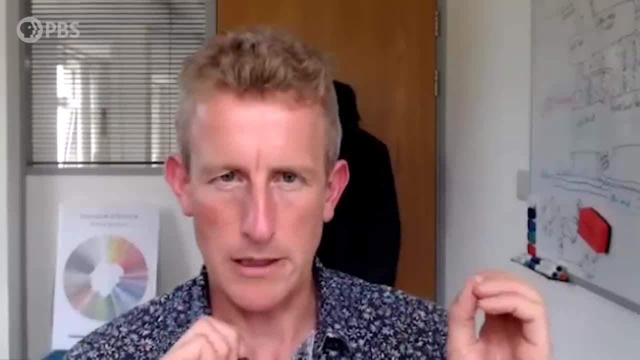 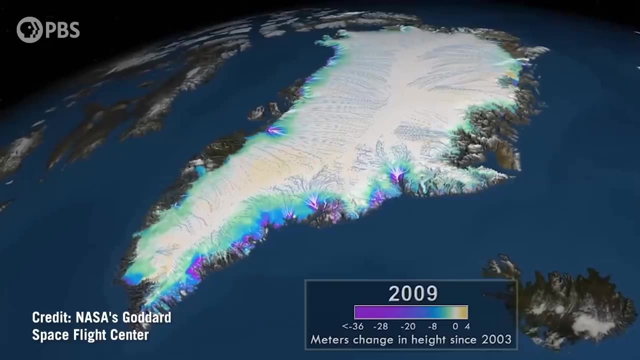 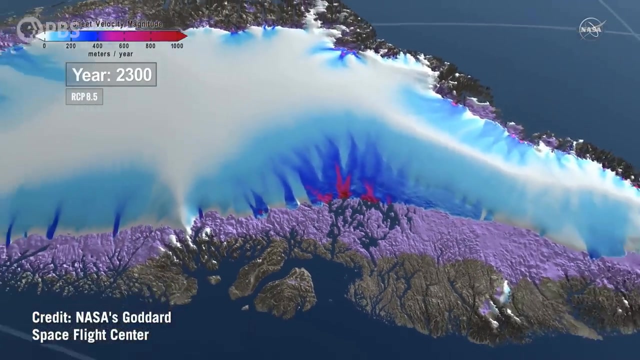 We're seeing accelerating melt of the Greenland ice sheet because of that extra Arctic heating. It's not just darker water absorbing warmth from the Sun. As Greenland's ice melts it exposes land which heats up faster than the more reflective ice in water around it speeding up the melt by 60% according to one recent study. Some of this is already happening. We're confident that the Greenland ice sheet can have a tipping point of where the melt and shrinkage of the ice sheet becomes irreversible. 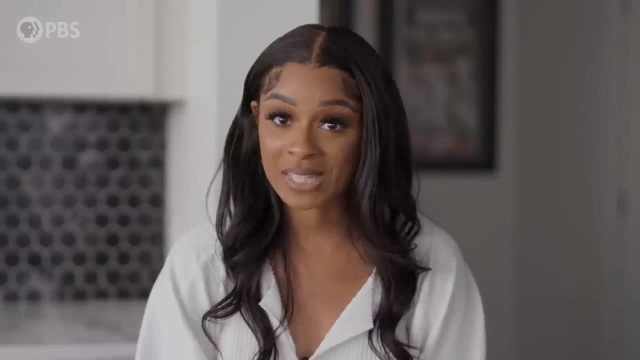 That could be close. Like very close. Tim recently published a study saying that the irreversible threshold could be just 1.5 degrees. 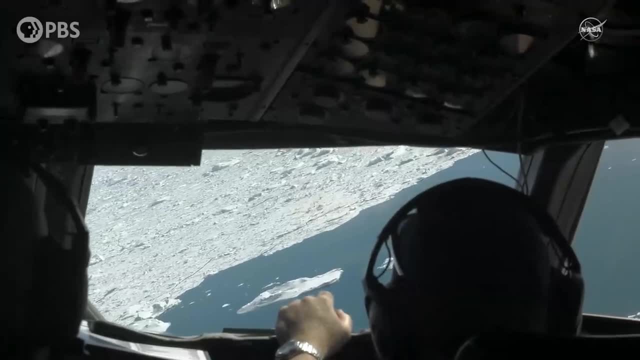 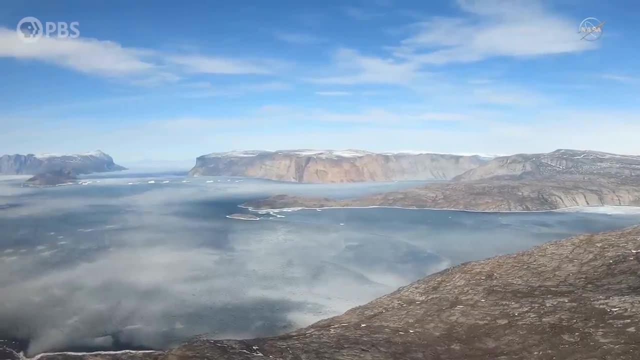 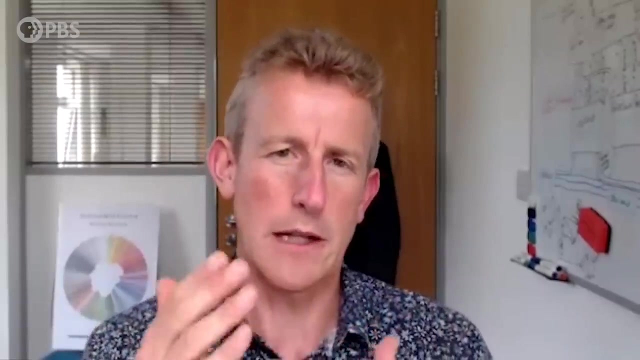 Certainly the ice melts and shrinkage is accelerating and has been for several decades now. And then the meltwater that's been in the ice sheet could be even more unpredictable. And then the meltwater that's been in the ice sheet could be even more unpredictable. that's pouring off Greenland, either side, into the North Atlantic Ocean, that poses a risk for what's called the Great Overturning Circulation of the Atlantic Ocean. 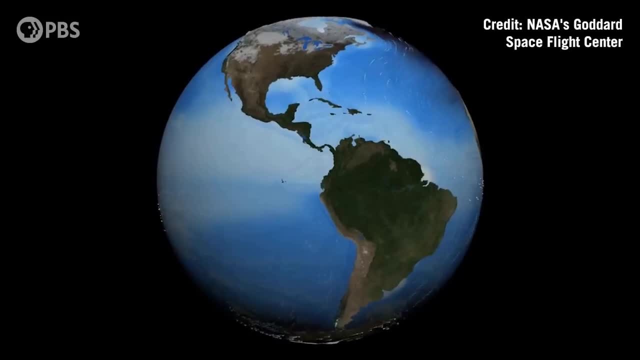 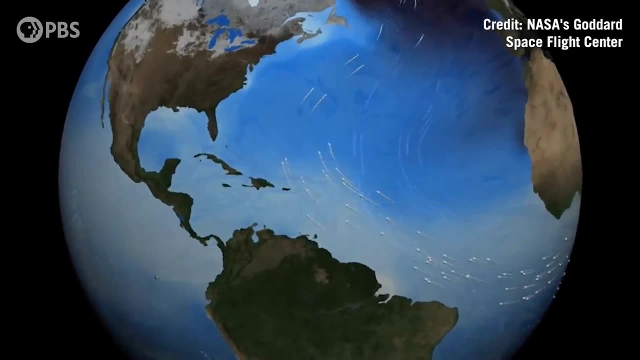 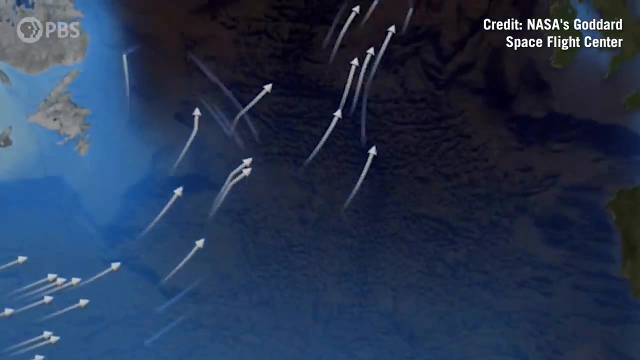 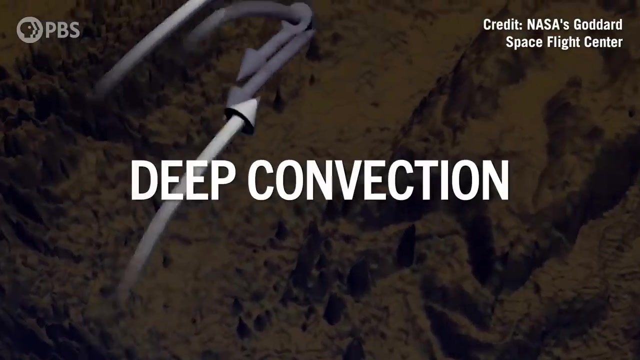 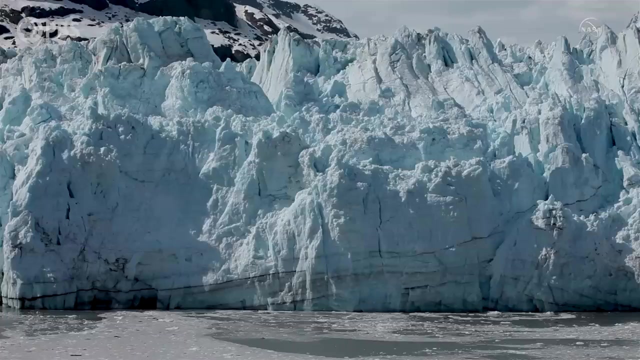 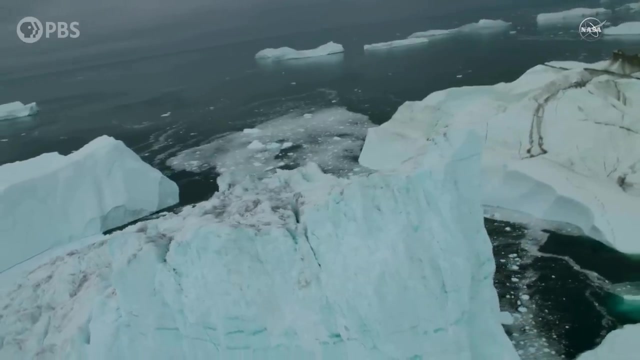 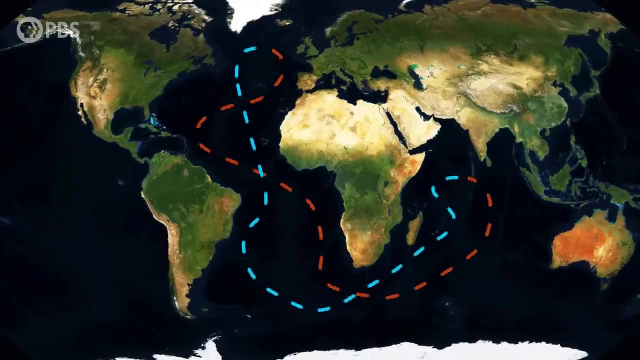 This is commonly referred to as the AMOC. It's essentially a giant flow of water that acts like a global conveyor belt, bringing heat from the southern hemisphere all the way up north to Greenland. Under normal service, the water gets cold enough and salty enough and dense enough to fall from the very top of the ocean all the way to the bottom, in a process we call deep convection, in the seas either side of Greenland. But if you add fresh water pouring off the Greenland ice sheet, you make the surface waters fresher, less dense, less prone to sinking to the bottom of the ocean. And this is certainly a factor contributing to some observed weakening of this Great Overturning of the Atlantic Ocean. Some calculations show that the AMOC has already weakened by around 15% in the last 50 years. 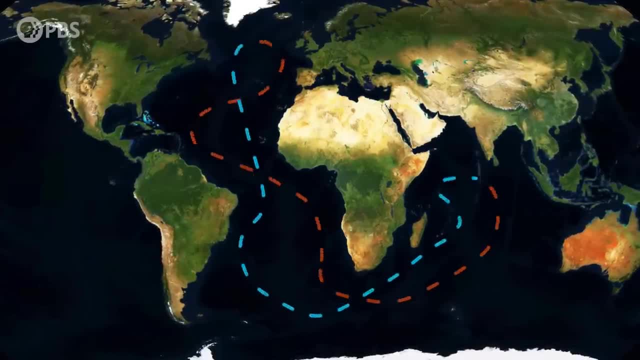 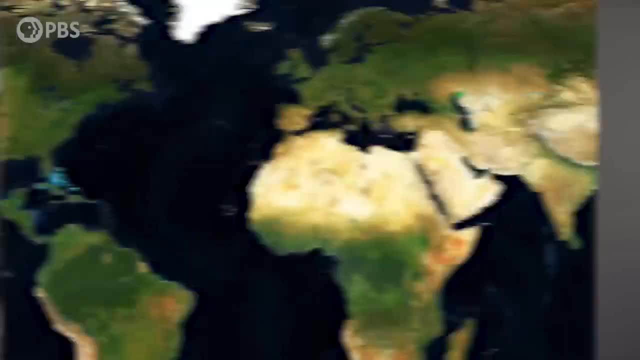 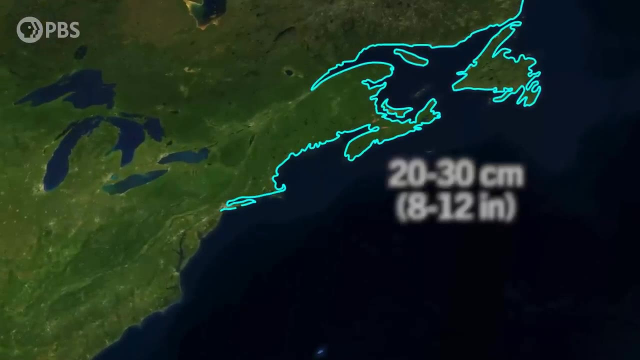 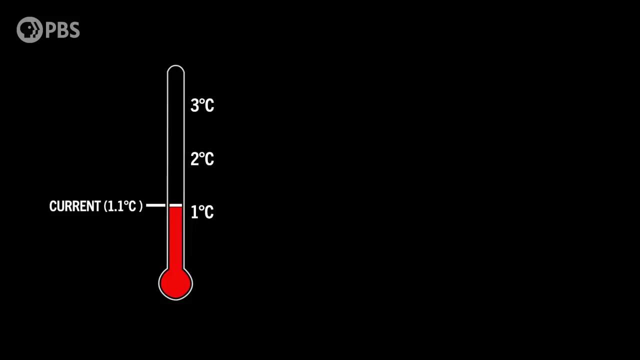 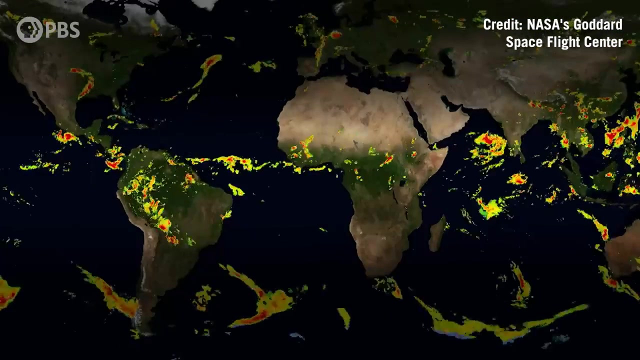 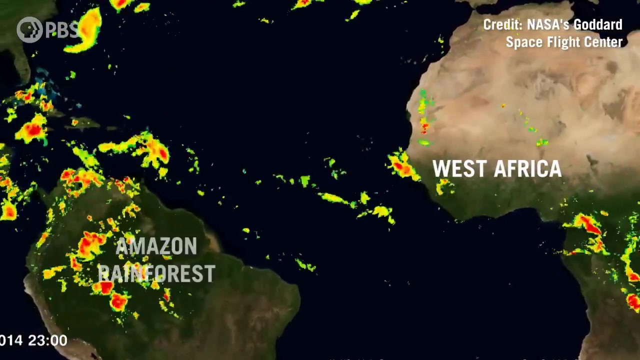 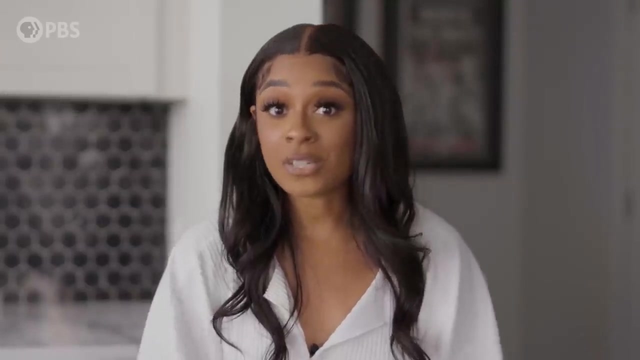 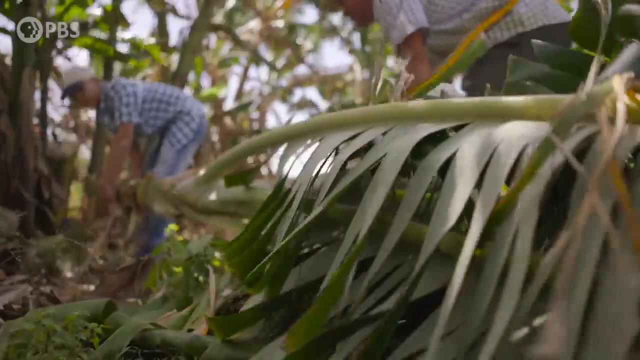 And scientists fear it could eventually slow to a halt, which would have extreme impacts on global climate as a whole. But even a partial collapse could plunge Europe into a mini ice age and raise sea levels along the northeast seaboard of North America by 20 or 30 centimeters. And models show that the tropical rain band that surrounds the earth would likely shift further south. Well, that means disrupting monsoon systems around the tropics, kind of near the Atlantic in West Africa on one side and South America, the Amazon region on the other, but also around the planet in India. Farmers around the world count on these reliable rain cycles each year. Changing their timing, location, or strength would disrupt the tropical rain band, which would likely shift further south. This could disrupt the livelihoods of over a billion people and complicate global food supplies as agriculture has to relocate and productivity is decreased. This could cause a large climate migration and weaken the food supply of over a billion people. Disrupting the rainfall regime and the monsoon over northern South America 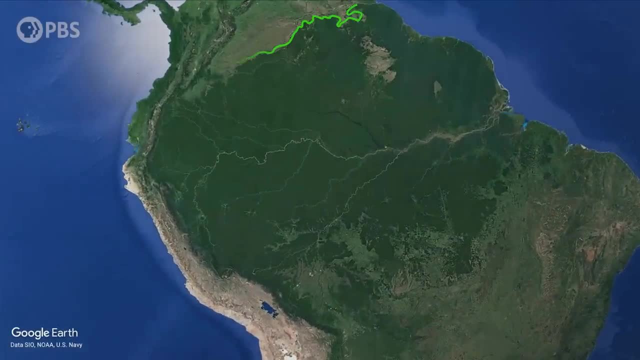 could be a big risk factor for the Amazon rainforest, which is definitely at risk of already 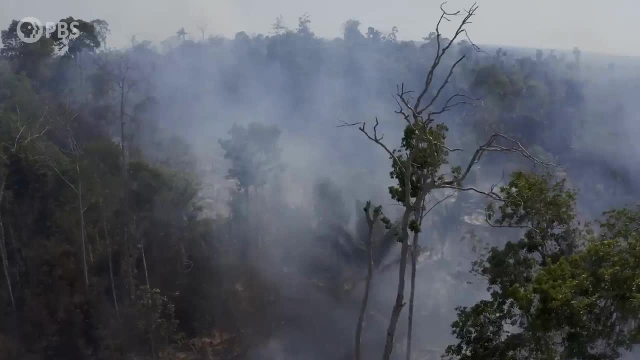 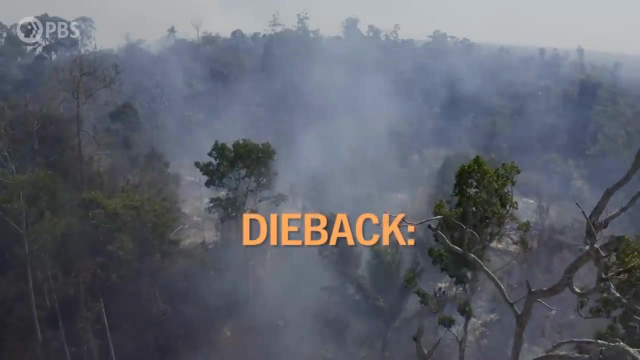 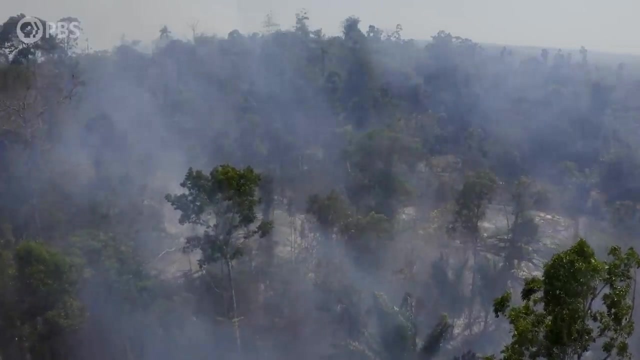 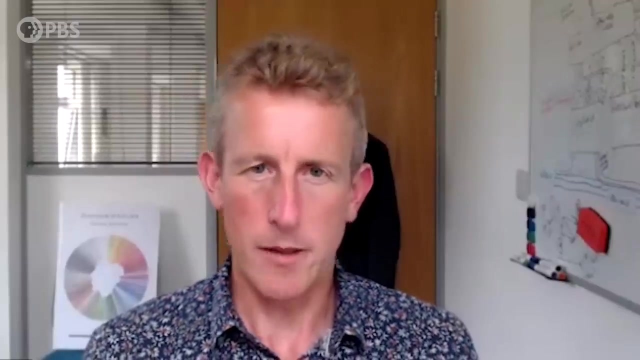 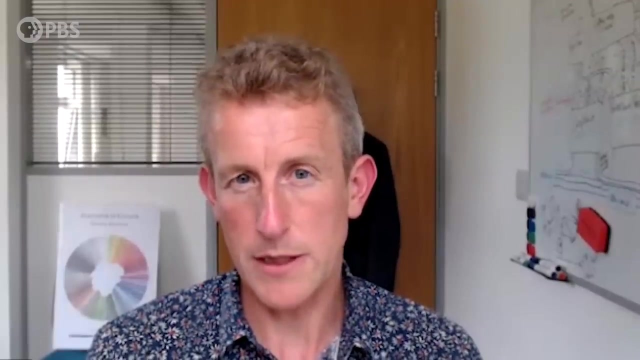 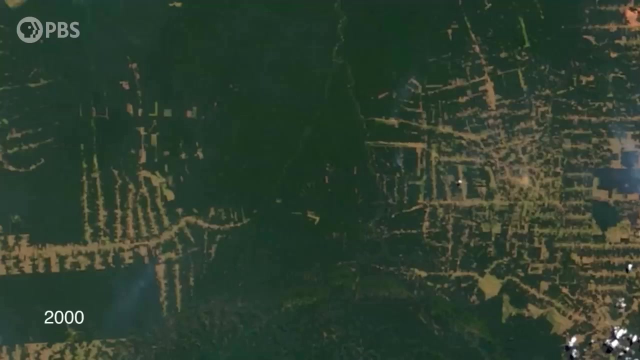 In fact, the Amazon experienced three one-in-a-hundred-year droughts between 2010 and 2020. These severe droughts contributed to massive diebacks, and for the first time in the forest's observed history, a large portion of it flipped from being a carbon sink to a net carbon source of greenhouse gas. So if this monsoon disruption amounts to further intensification of the dry season, that's the thing that could risk a more widespread dieback of the Amazon forest that then becomes self-propelling because the Amazon recycles its own rainfall back to the atmosphere. You take the trees away and you reduce the recycling that tends to take more trees away and so on and so forth. 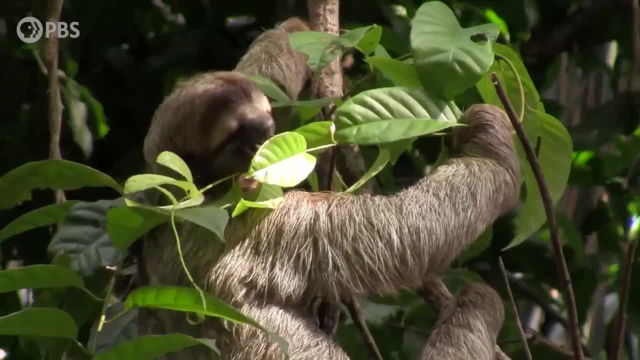 Well, we don't want that to happen for various reasons because we don't want to lose perhaps the greatest harbour of diverse life on the Earth's land surface. 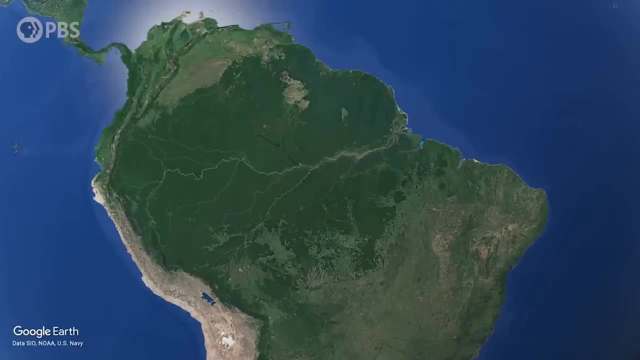 Okay, that's not great. But now let's head back to the ocean and continue south. If the Atlantic overturning is weakening, we're leaving heat behind in the Southern Ocean 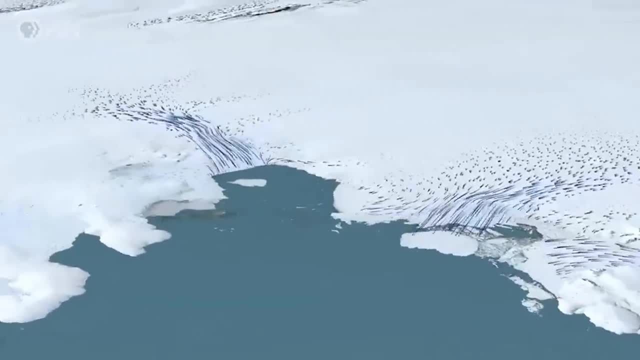 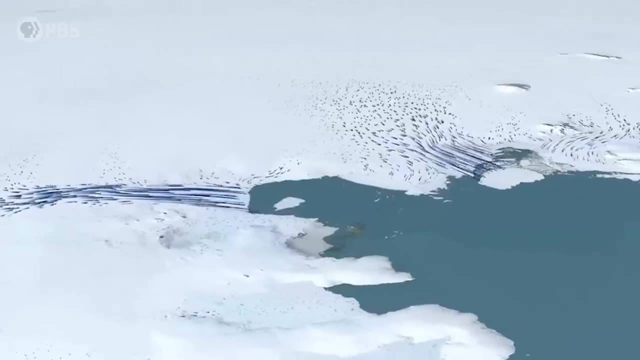 and heating up of the Southern Ocean is the biggest threat factor for the Antarctic ice sheets. And as we've covered in a previous episode, we know that the West Antarctic ice sheet is already destabilizing and could be close to a tipping point without added warming of a weakened area. 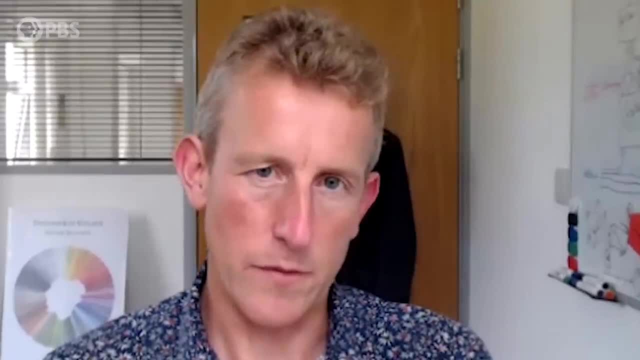 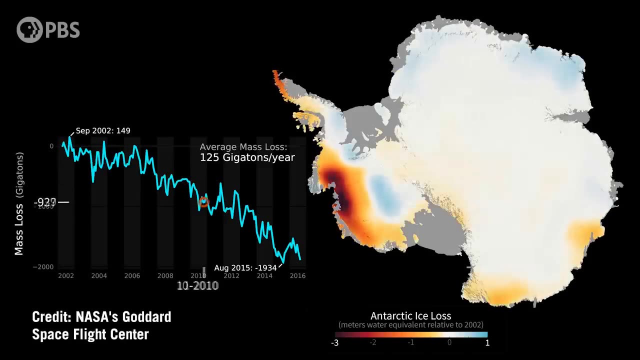 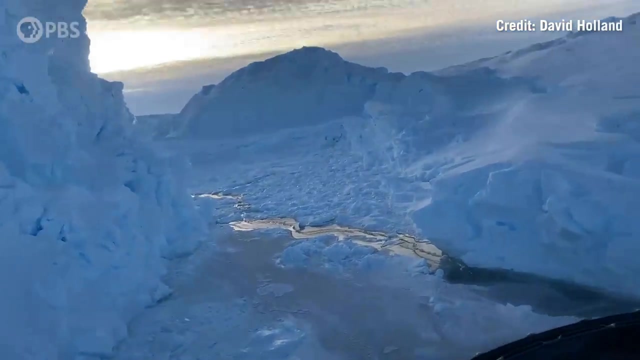 And yeah, if you heat the ocean up, that's the big threat factor to further accelerating the loss of that ice sheet, but also a threat to the bigger East Antarctic ice sheet. You start to trigger a retreat of the glaciers that causes the glaciers to flow out faster, so it becomes self-propelling. So that's a lot of bad news, isn't it? 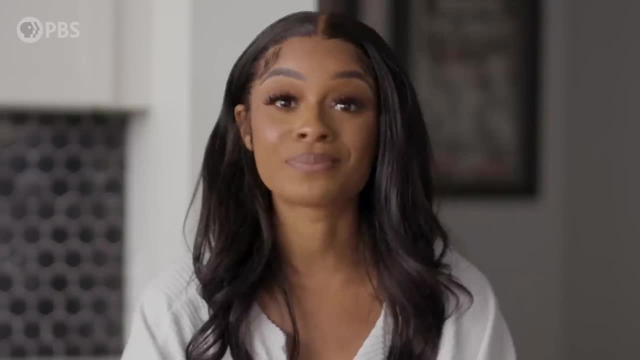 Well, yes, Tim. Yes, it is. So what's next? The permafrost is thawing. 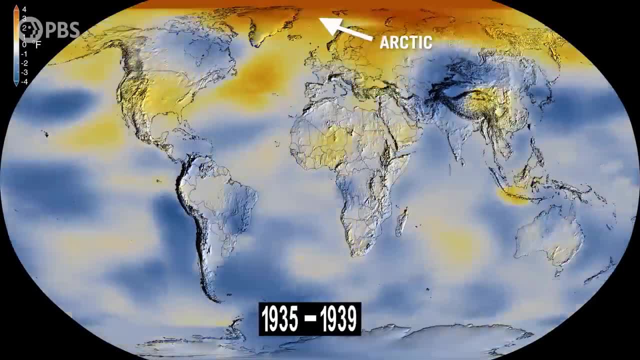 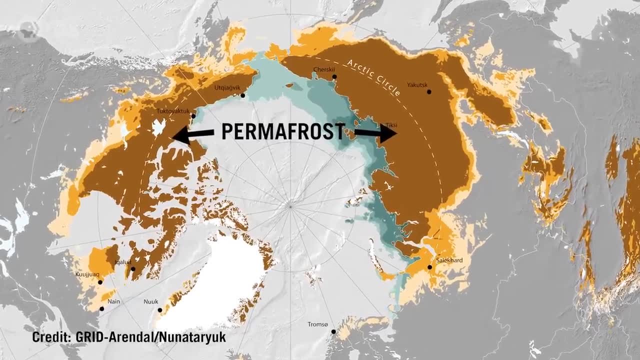 And the permafrost is thawing at an accelerating rate, not least because the whole Arctic is warming at an accelerating rate. And the permafrost is important because it's a really big frozen store of carbon. 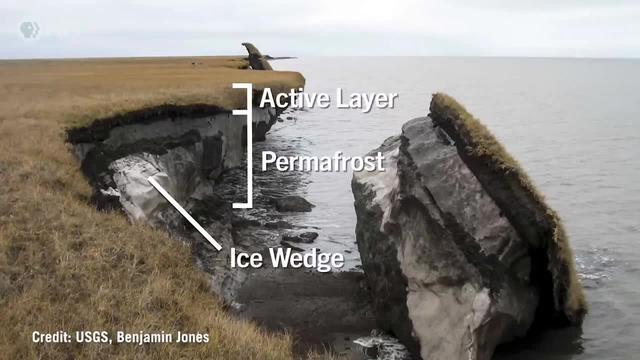 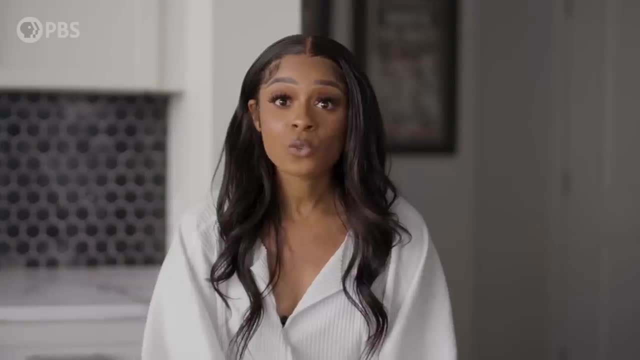 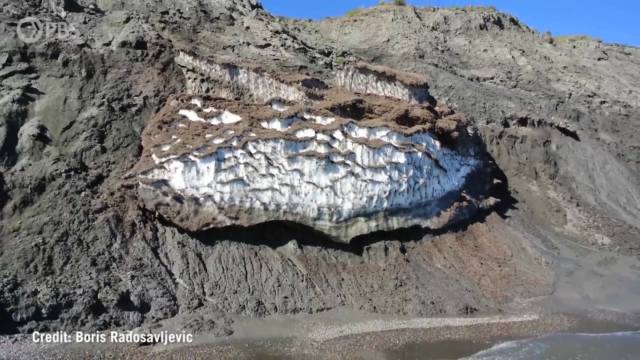 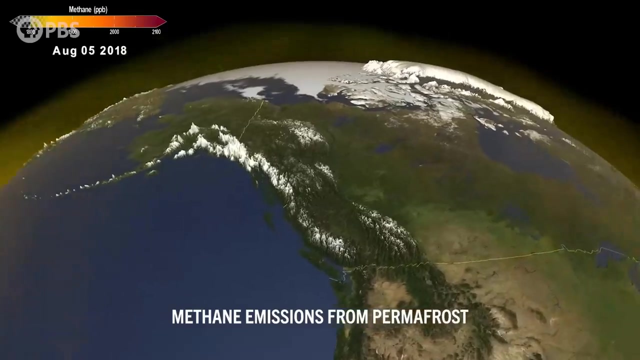 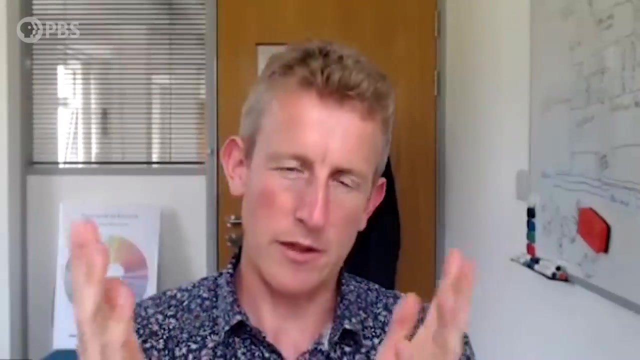 Really quickly, permafrost is land that's frozen year round and has been for a long time. When it's frozen, there's no tiny bugs to eat the organic matter it contains. So the massive stores of carbon are safe. As you start to thaw it, well, the permafrost is thawing. And that's a lot of carbon because bugs are basically going to work. They might be the kind of bugs that turn some of that carbon into methane, which is a far more potent greenhouse gas than carbon dioxide. Meanwhile, other bugs are turning it straight to carbon dioxide. 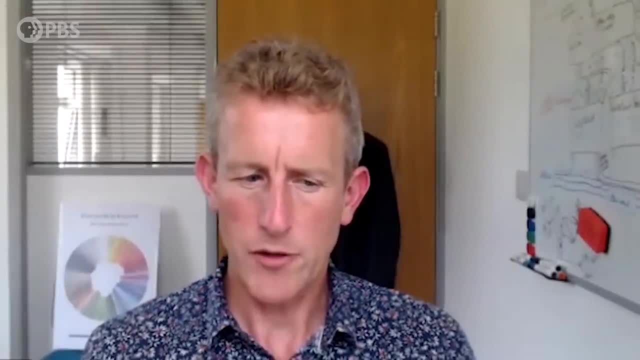 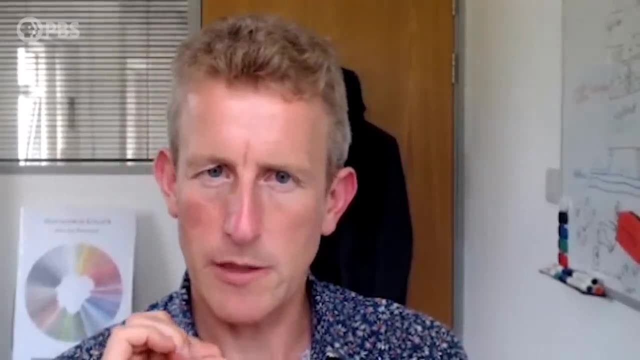 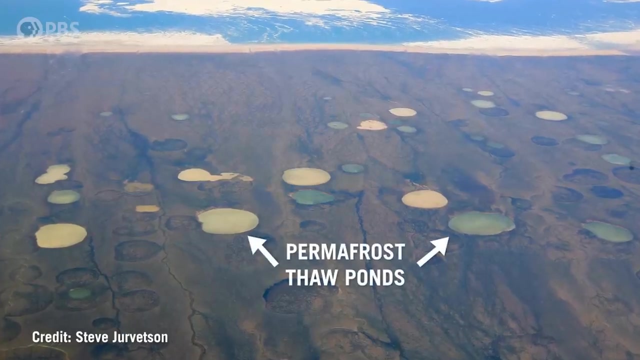 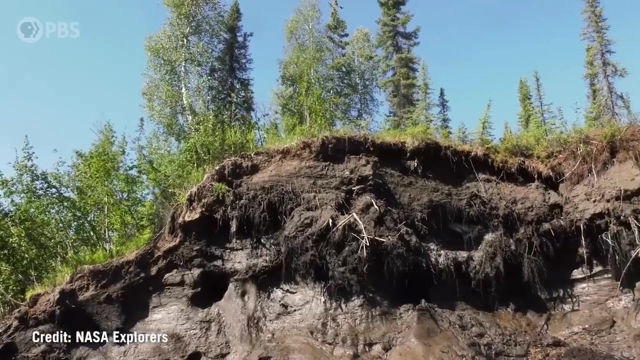 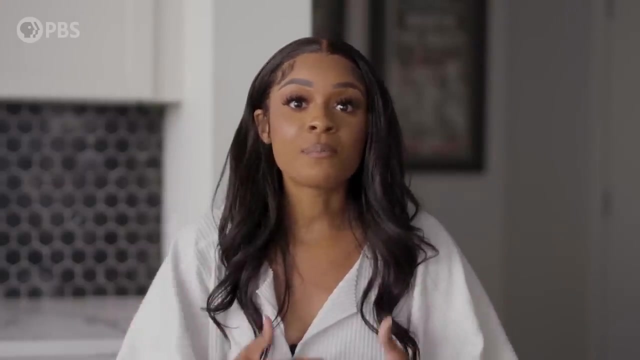 Both of those things are being added to the atmosphere, adding to warming. But on top of that, when bugs eat carbon that's coming out of the deep freeze, they release heat just like tummies release heat when we eat food. Releasing heat in that permafrost column can thaw more of the permafrost, giving them even more food to eat to generate even more heat to thaw even more permafrost. And that means a true tipping point of a sort of self-propelling breakdown. And to put that into context, we're talking about hundreds of billions of tons of carbon dioxide and 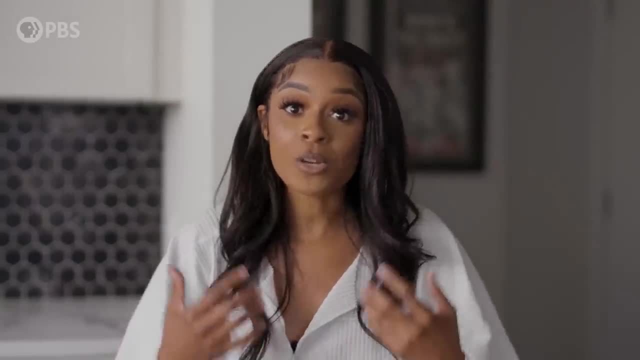 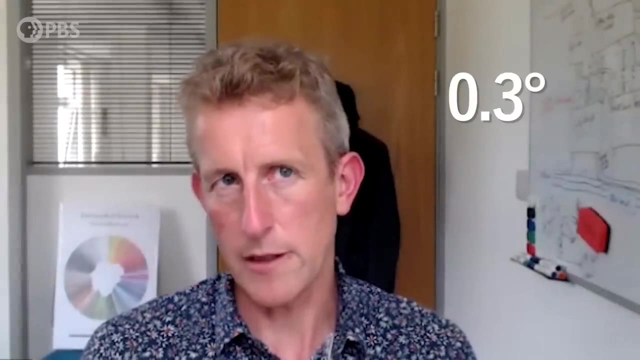 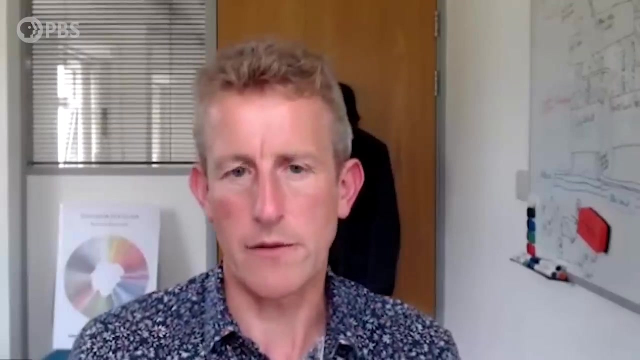 methane that could be released from the permafrost, which would add measurably to global warming. By point one, two, three, a degree C and adding to the overall risk and adding to the likelihood of tipping some of those other systems if they haven't gone already. 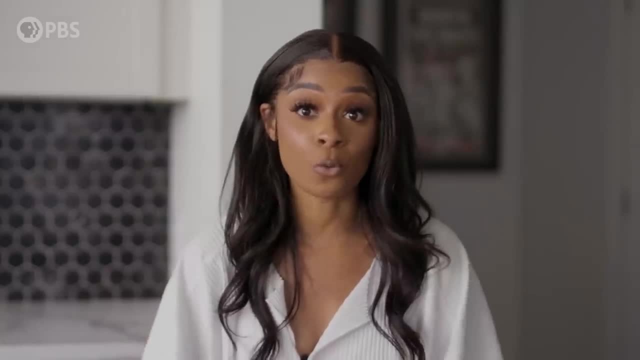 We're clearly talking about a very different future of the world here. And there's one tipping point that has likely already been reached. 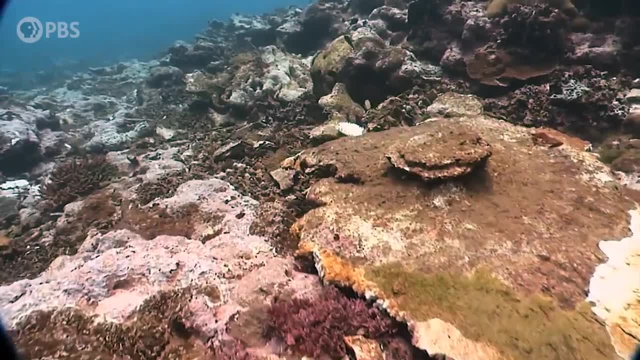 There are still lots of living coral, but it's being bleached so quickly by hot ocean water that it may never exist in the way that it did just a decade ago. 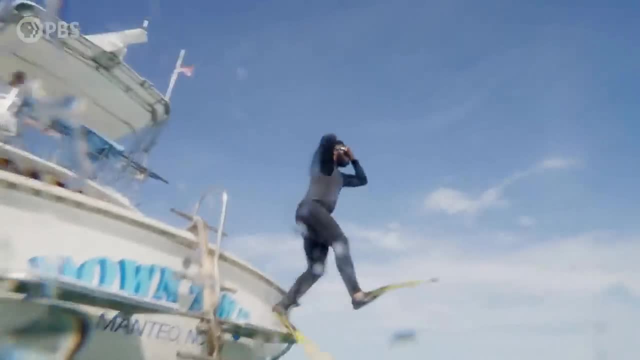 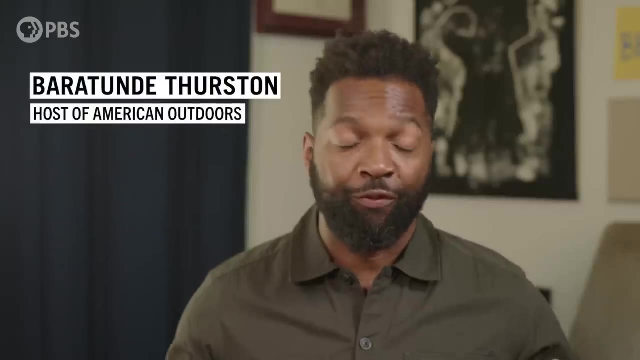 So I asked Baratunde, K. Thurston from American Outdoors Understory, what swimming over a reef is like and what the loss of coral reefs means to him. K. I felt like I was flying across this underwater mountain range, but unlike any mountains I'd ever seen. 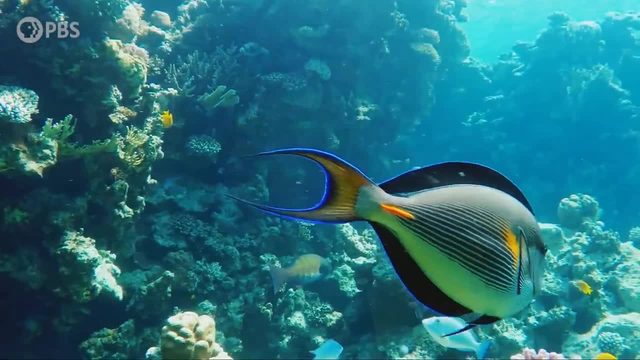 It was like mountains made of hyper colors and there were fish flying around too. And they were saying what's up and I was saying what's up. 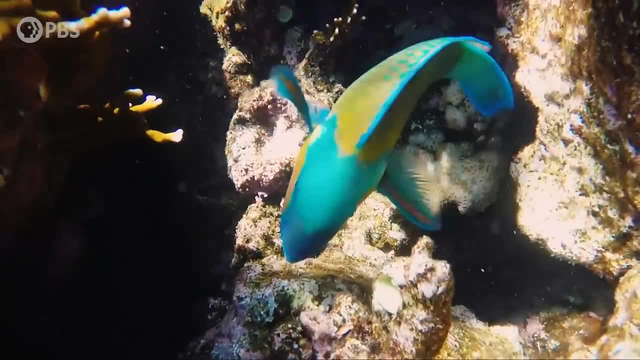 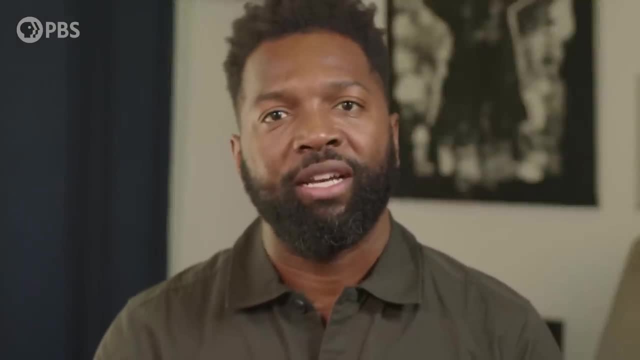 And the idea that they wouldn't have a home that all of that life would be dead, that all of those colors would be bleached out. I'm really, really sad about the prospect that we will lose a piece of ourselves when we lose these coral reefs. 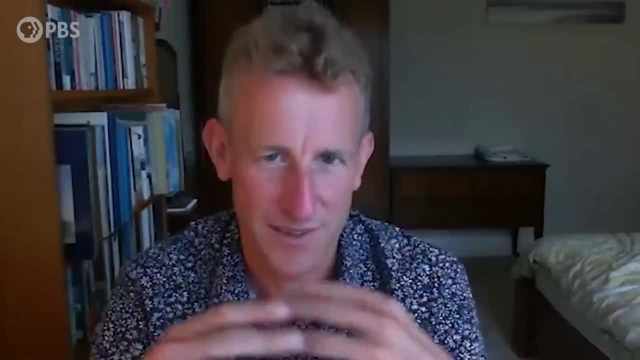 It takes a while for the consequences of passing a tipping point to fully unfold. It can happen a lot quicker for coral reefs as we've seen with iconic bleaching events across the Great Barrier Reef and the like. 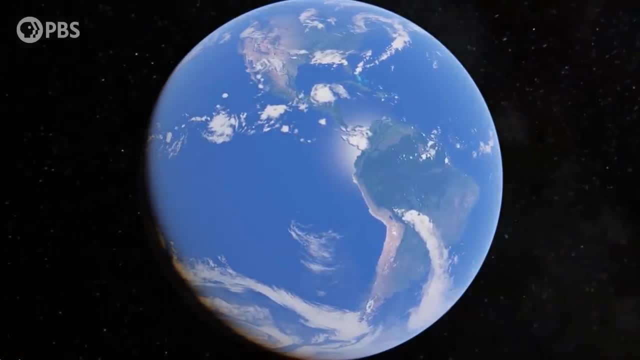 So what will the Earth actually look like if we reach these tipping points? Well, it's pretty dramatic. 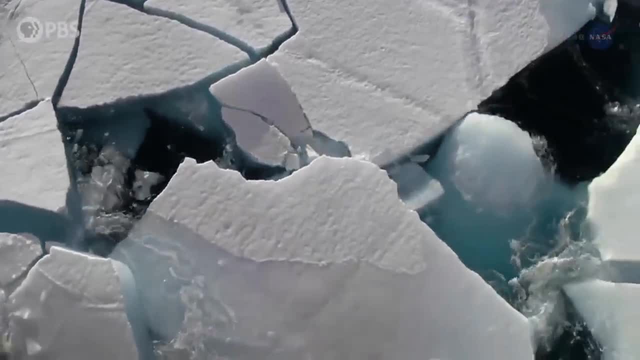 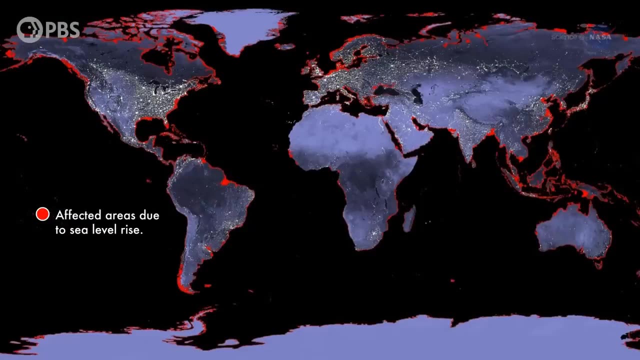 With melting ice from the Antarctic and Greenland ice sheets, Tim says we're already committed to 10 meters of sea level rise, which will essentially redraw the coastlines of the world and displace about a billion people. 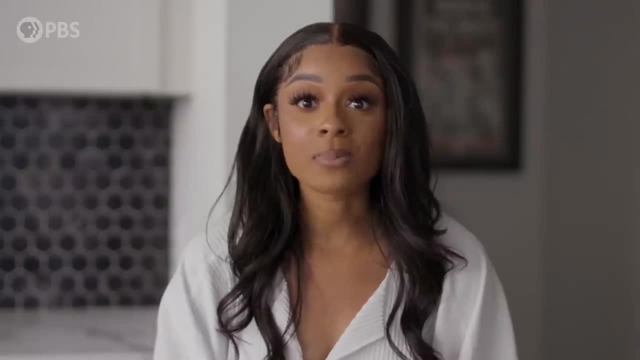 The Amok collapse is fascinating. A total collapse could actually mean something 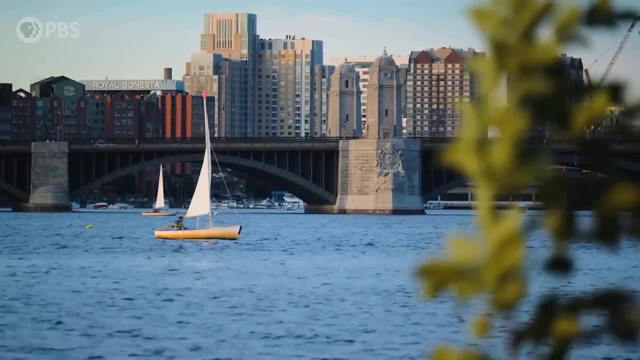 of a mini ice age in parts of Europe, as well as significant sea level rise along the northern seaboard of the US. 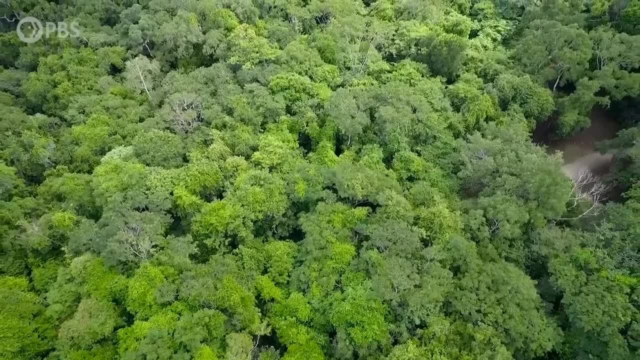 Amazon dive back would turn much of Brazil from a rainforest into a very different ecosystem, 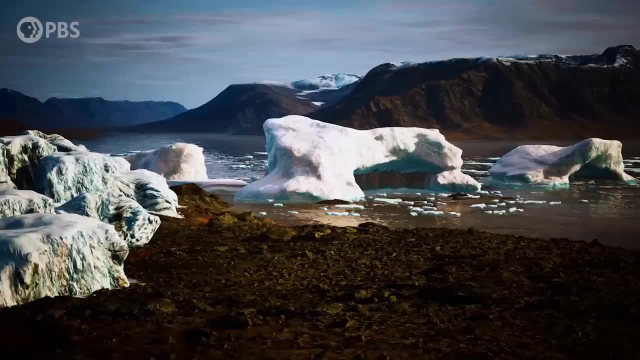 potentially grassland or even drier. And while Greenland ice melt would cause massive sea level rise globally, 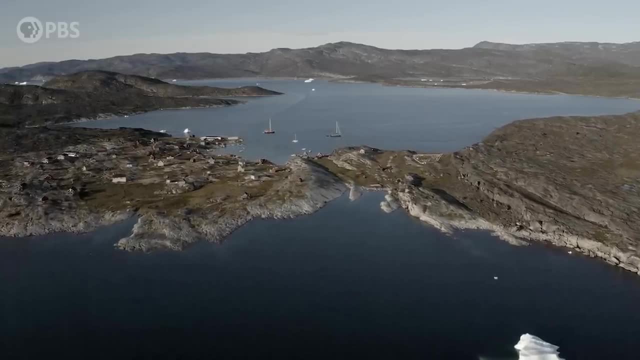 locally, there will be more room for agriculture and people as the ice exposes more land. As melting continues, places like Siberia and Northern North America that currently have very shallow permafrost could see larger and more dense forest in the long run. 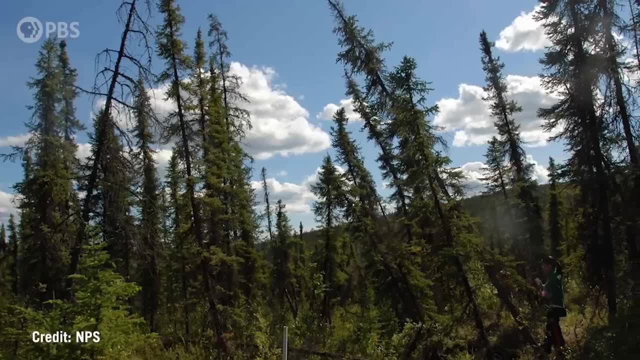 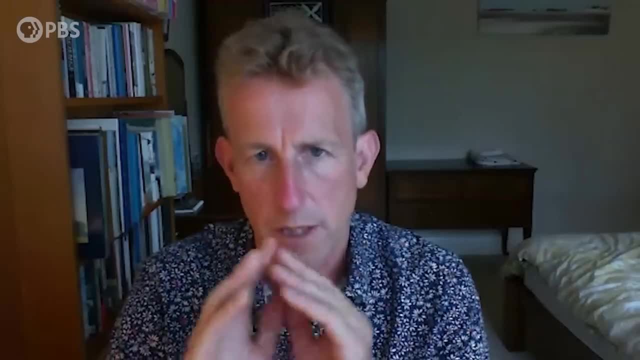 This has got profound implications for the kind of every other living thing and the future trajectory of evolution. 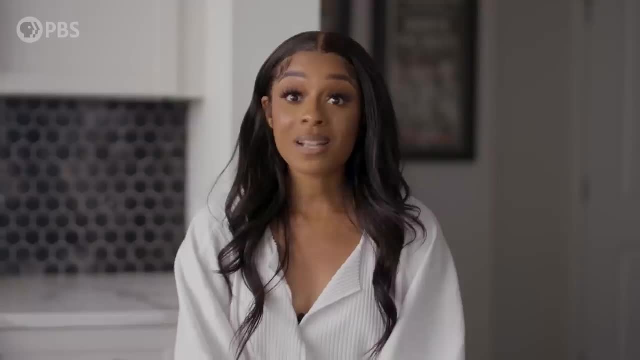 So, it's a hell of a legacy for us to be leaving. But this isn't written in stone and there's still time to stave off the worst case scenario. 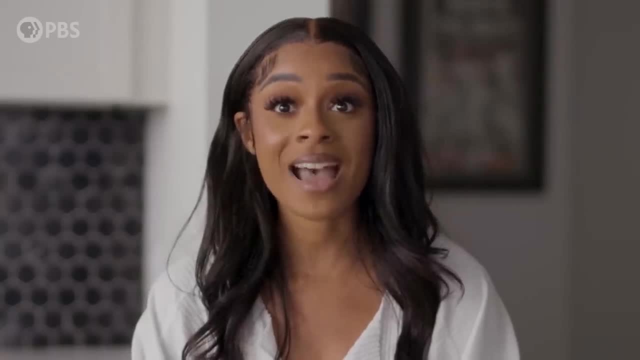 Still, we know some adaption will have to happen and Tim has an idea for mitigating the impacts of those tipping points that we just can't avoid. 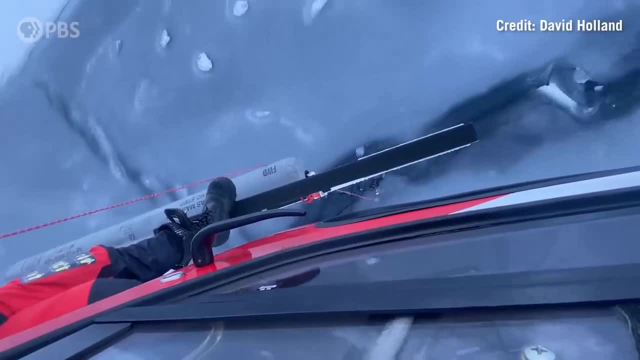 We know now, even just directly from observational data, we can see systems losing stability before they hit a tipping point. 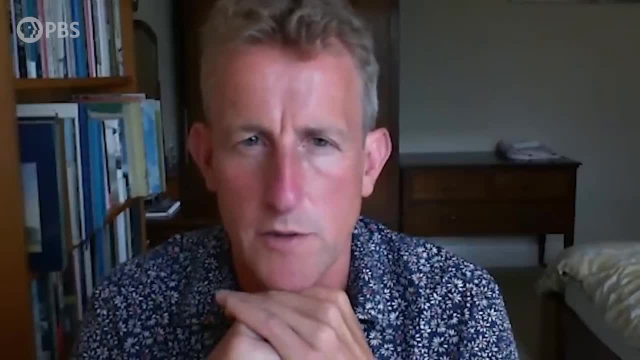 So, if we have an effective tipping point early warning system that's telling us about some of the most impactful biggest risks that are coming, 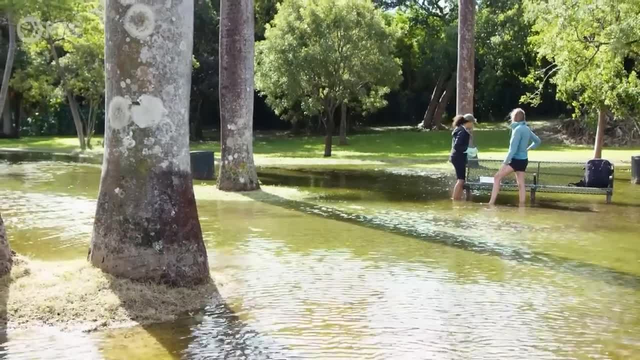 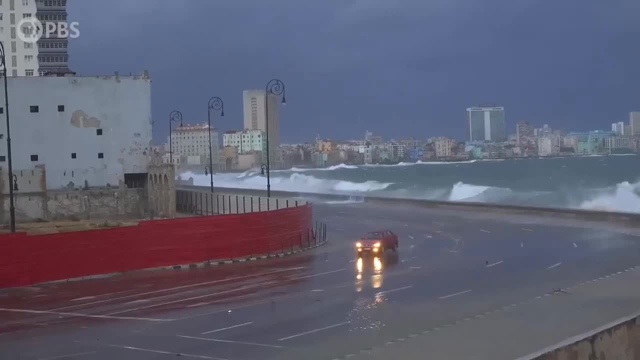 in simple terms, forewarned is forearmed. I mean, we can use our resources wisely to reduce the damage, even for the unavoidable stuff. 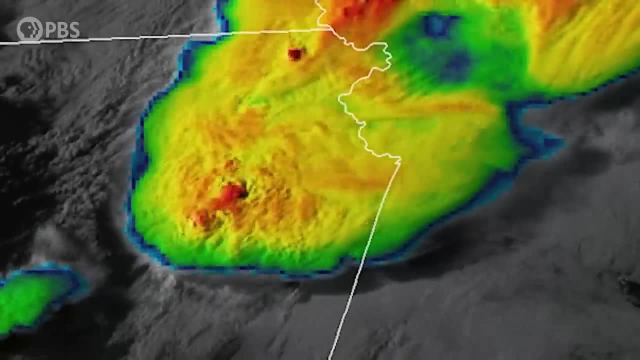 There are examples already in use for earthquakes, tornadoes, hurricanes, and even wildfires. 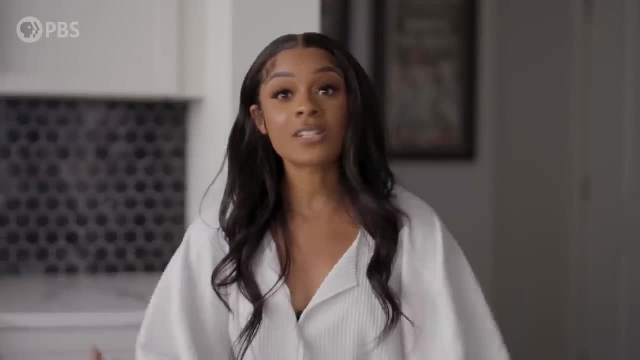 But does a planet scale warning system seem possible? I'd love to hear from you. 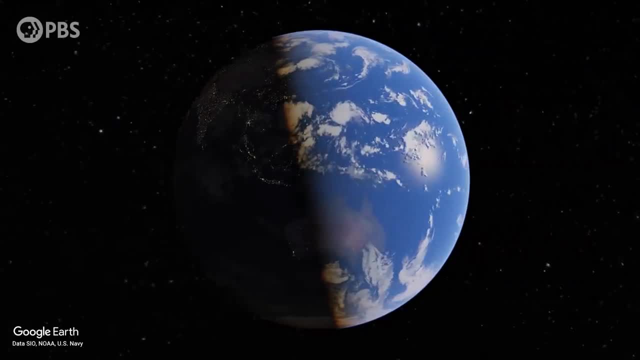 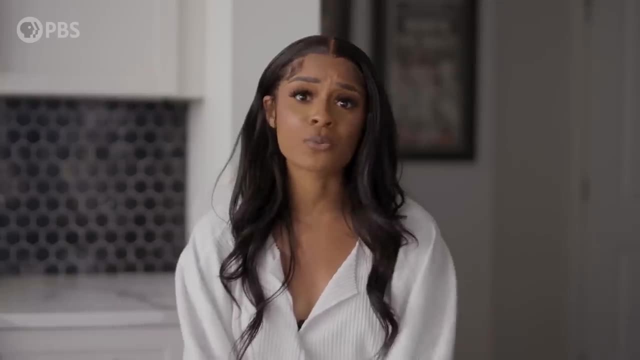 What would it take for us to make the changes needed to stop warming at 1.5 or two degrees? And remember that even though these are major scary changes 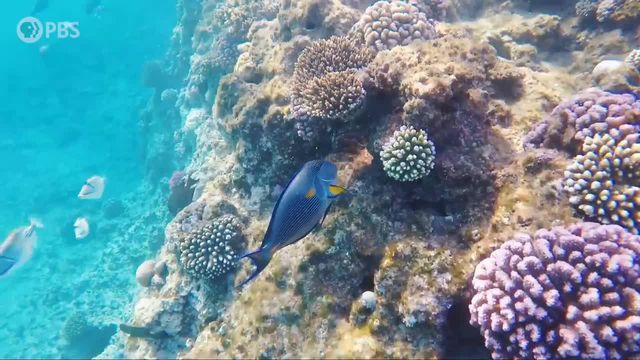 we're talking about, there's still so much beauty in the world to enjoy. 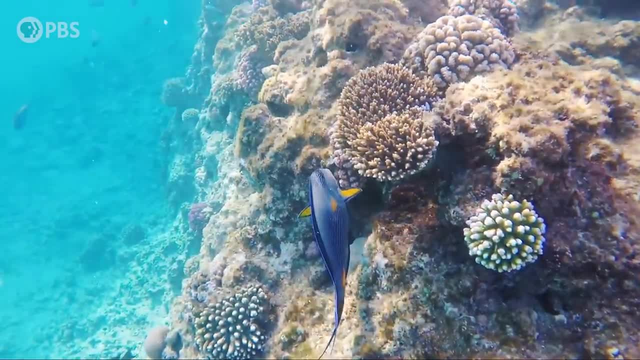 Just think of all the wonderful corals that are still thriving. 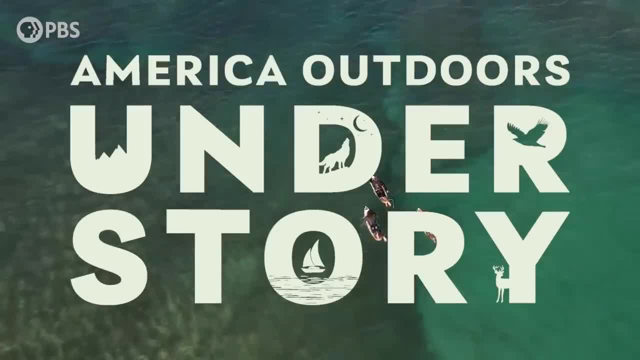 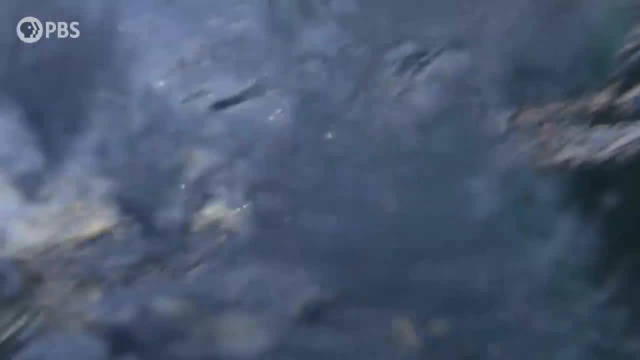 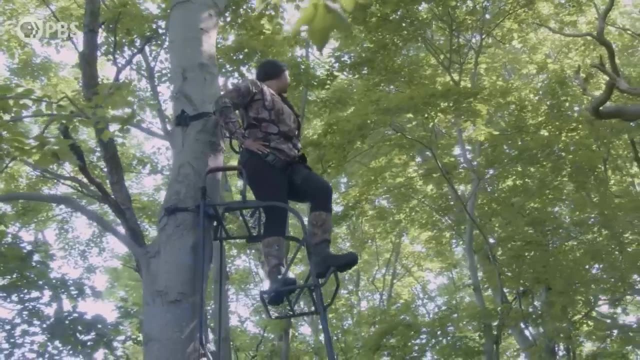 I'd love to love the newest show in the PBS family, American Outdoors, Understory with Baratunde Thurston. From episodes on surfing scientists combating climate change to the scorched, desolate beauty of Death Valley, this show explores our passionate and complex relationship with our natural world. Check out the link in the description and tell them Weathered sent you.